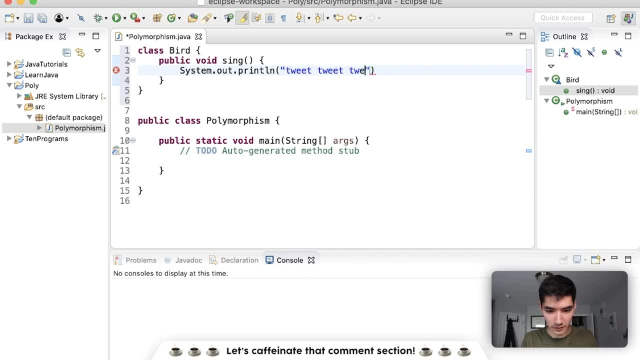 will go tweet, tweet, tweet, tweet. Now, if we create this bird object in the main method, we can do bsing And we'll see the code inside of that sing method run Now. this is one form of the method sing, But 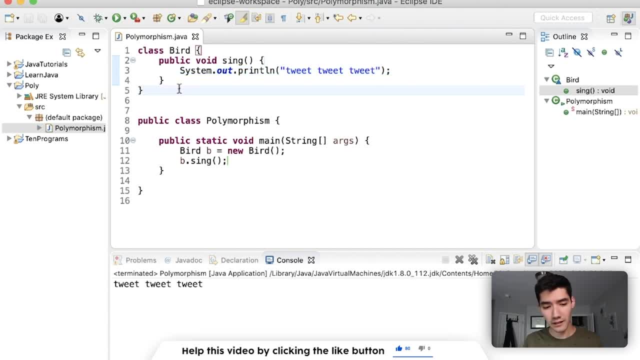 we want to get into many forms polymorphism. This comes into play when you have a class that's related to it that also has that same method. Let's use inheritance to create another bird that has the same sing method. Now, what's a subtype of a bird? What's a kind of bird? 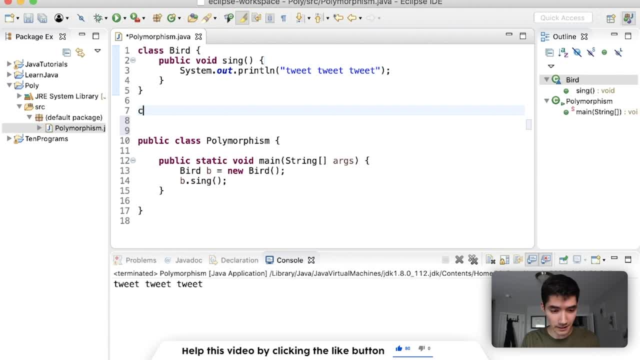 We could do a robin, So we can say that we have a class robin like this. Now, what we could do is copy and paste this in here, Or we could assume that it already knows how to sing the same from the bird by typing: extends bird. This means every time we make a 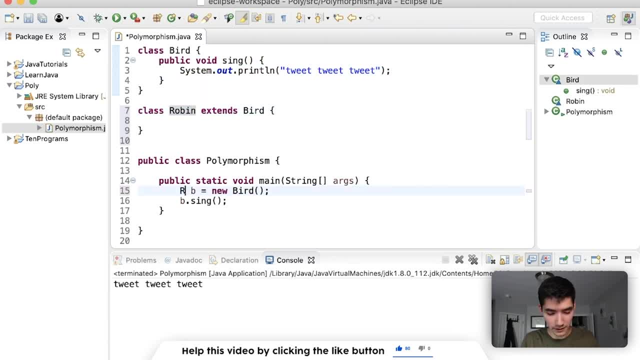 robin. it knows everything inside of the bird class. So if we do robin b equals new robin. it can still know how to sing. And if we create another bird, for example let's say pelican- I don't know what sounds pelicans make, but it is a bird- So we can extend bird. And if we do, 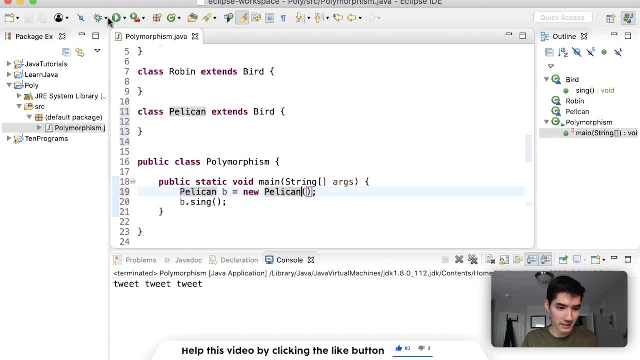 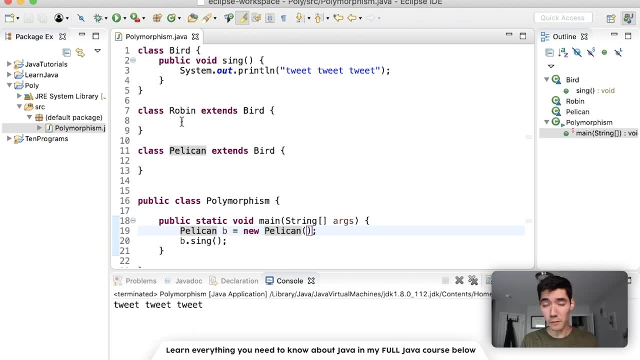 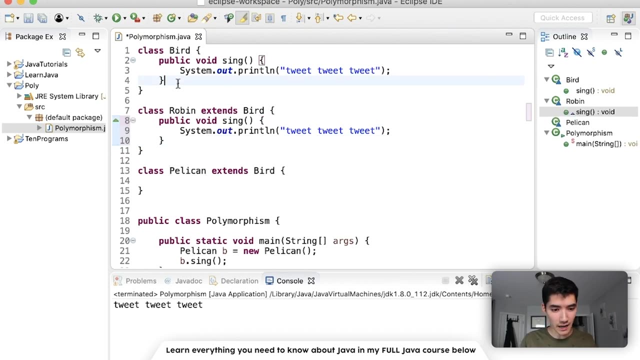 pelican here. it'll be the exact same, It'll sing the exact same, But this isn't exactly accurate. All birds don't go tweet, tweet, tweet, you know. So what we can do is create its own sing method that will act a little differently based on what kind of bird it is. So I just copied and pasted. 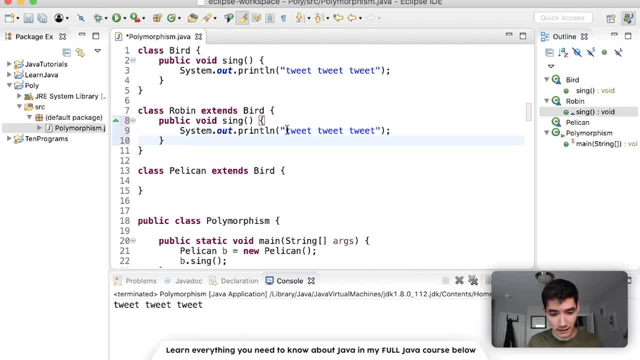 the bird sing method And then I'm going to copy and paste the bird sing method And then I'm going to paste it into the robin sing method And maybe the robin goes twiddle, twiddle dd. Yeah, let's say the robin goes twiddle dd. Technically now, this robin class knows a method called sing, but it